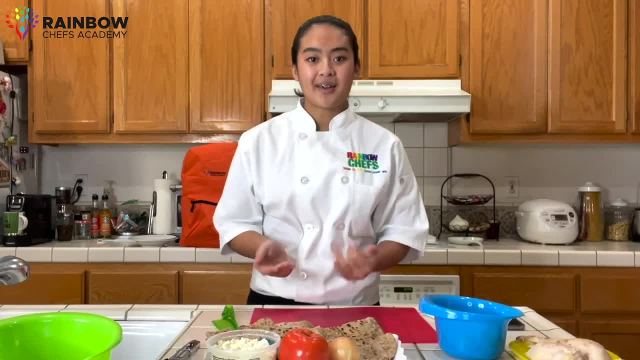 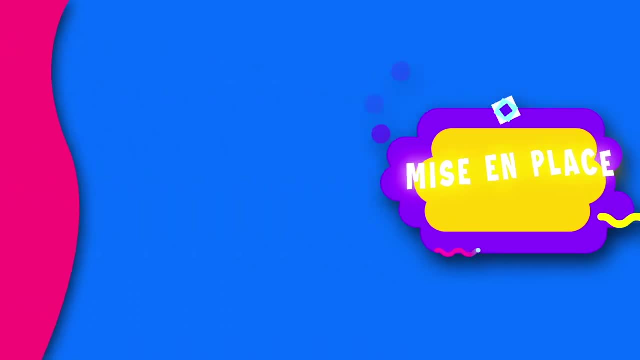 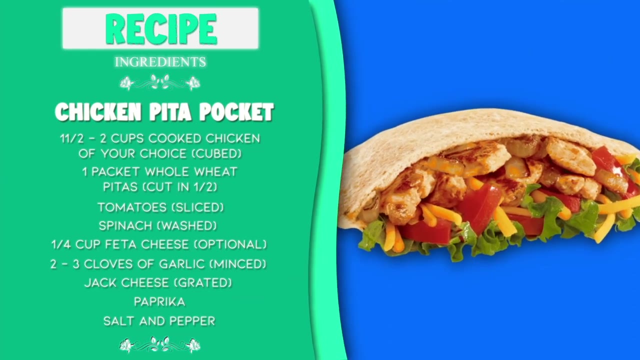 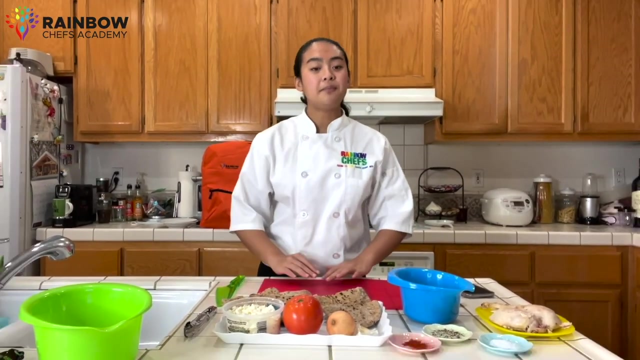 and with soap. That way, there's no bacteria in our food when we're cooking. Be right back Now that our hands are clean. we're going to now start preparing our mise en place, which is French, for everything in its place. So in front of me we have chicken breast. 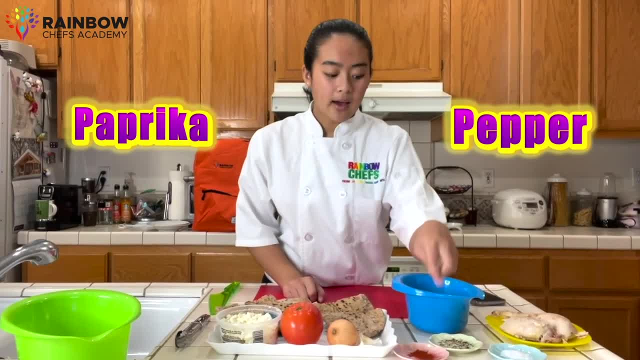 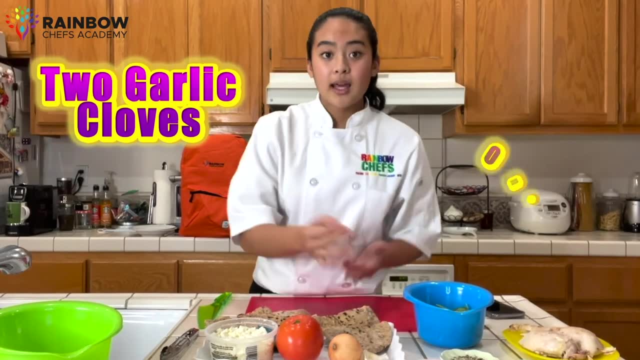 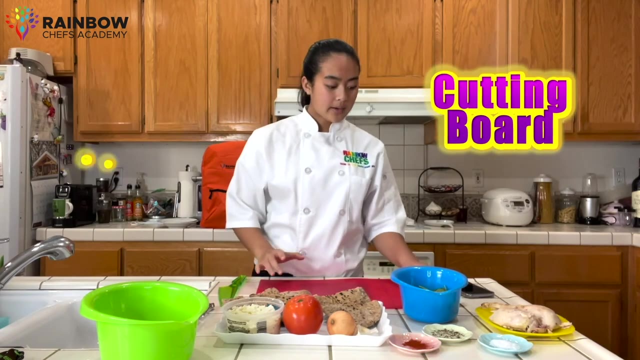 which is pre-cooked: salt pepper, paprika, fresh spinach, pita pockets, whole wheat, feta cheese, tomato onion, two garlic cloves, and for our materials we have a medium to small mixing bowl, some tongs, a chef's knife, a cutting board and a spatula. 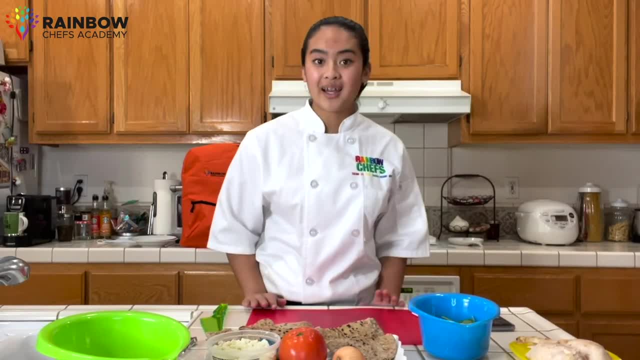 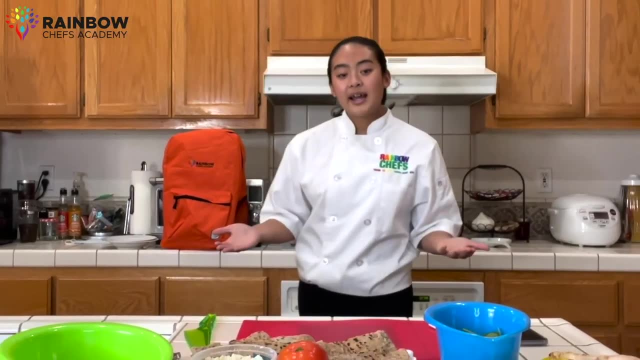 Hmm, are you wondering where we get all these materials to start cooking in the kitchen? Well, I have a tip for you. Right behind me, I have our cool new rainbow chef backpack. Everything inside it contains materials that we'll be using throughout this channel for every. 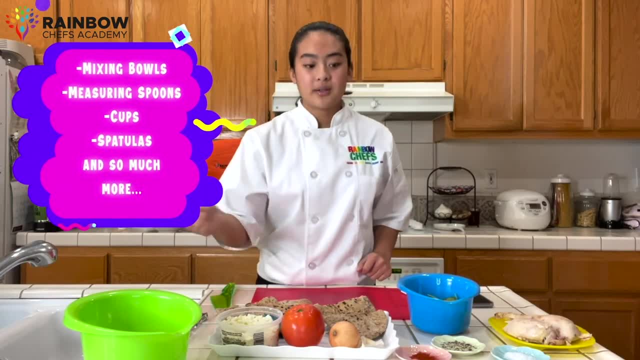 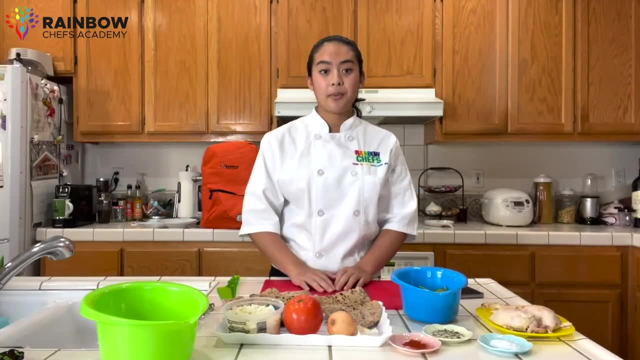 single recipe, such as mixing bowls, measuring spoons and cups, spatulas and so much more. If you would like to purchase, go check out our website. To start making our chicken pita pockets, I began by cutting our pita pockets in half and separating them so that way it's similar to a 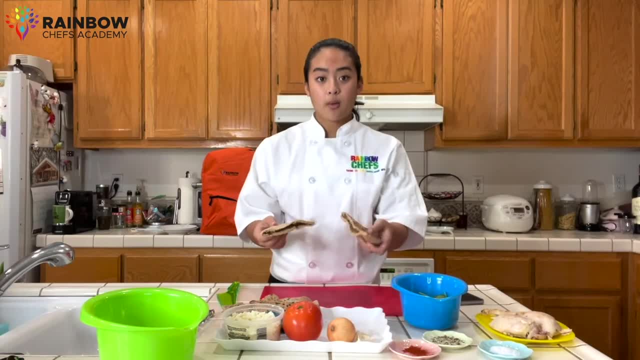 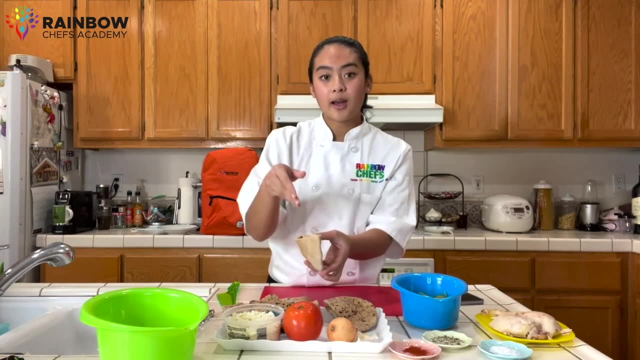 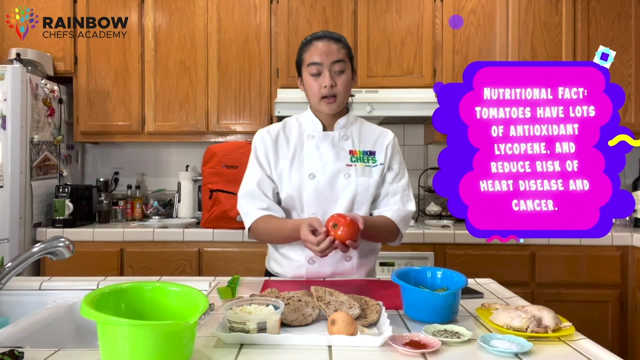 little pocket. A lot of them will come in stores, will come as a circle, but you simply just cut them in half and split the two centers, so that way you're able to stick our chicken and veggies inside later. Next, we're going to start by dicing our tomato. So, to begin, we're going to start by 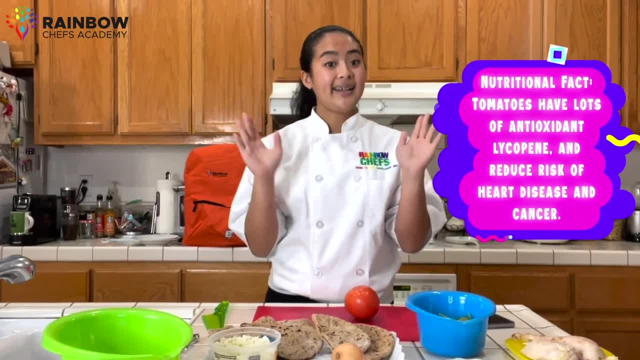 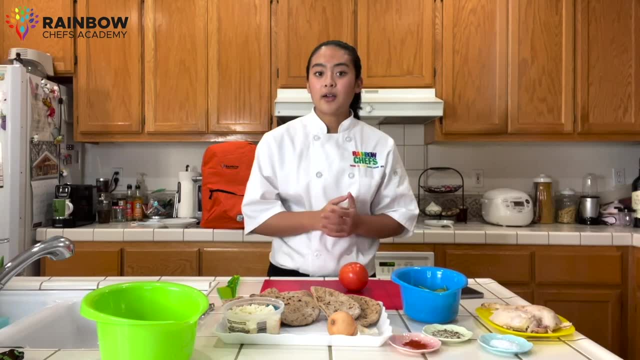 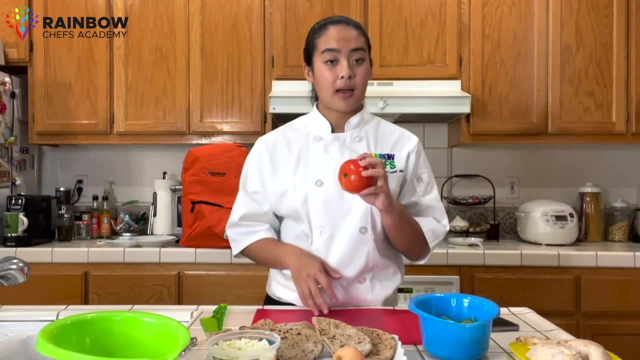 cutting off the stem part. Before we cut anything, I'm going to teach you the proper way to hold a knife and hold your veggies while cutting So with your left hand. depending off if you're right, dominant or left-handed, you are going to grab it with your claw. I am right-handed, so I will be using my left hand. 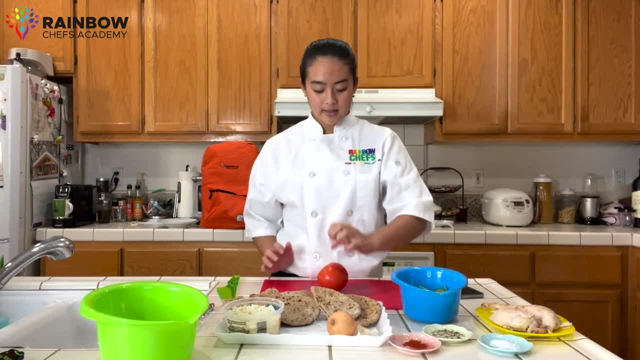 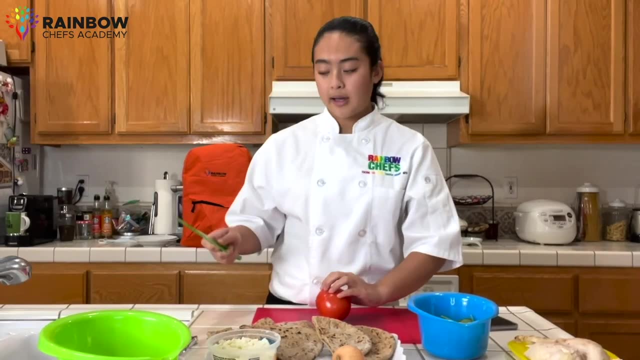 but a claw is basically when you pinch in your fingers just like this to hold your veggies to avoid your fingers to be cut while you're cutting with your sharp chef's knife. Now, while holding your chef's knife, you're going to please your pointer finger. 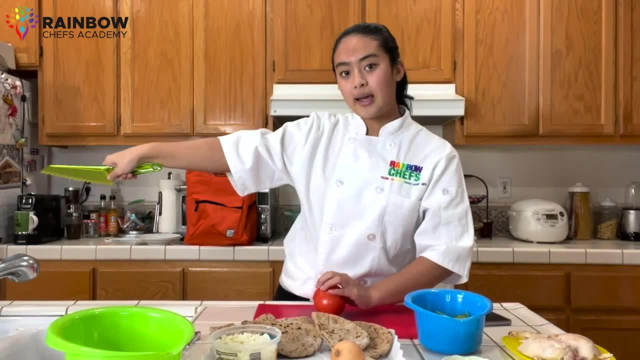 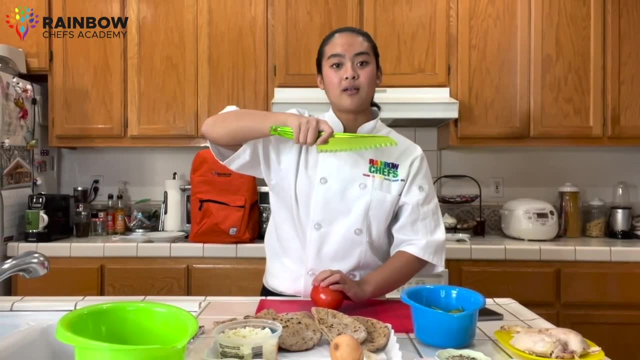 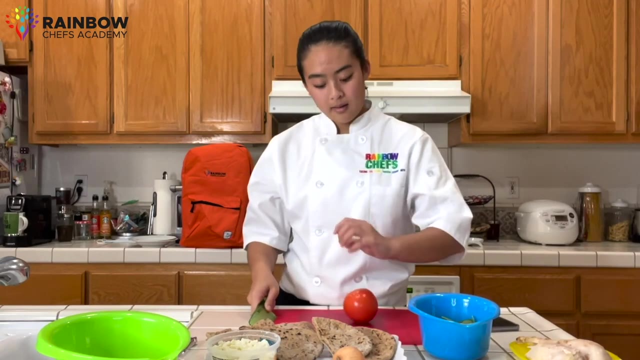 and your thumb You're going to pinch the end of your knife, just like this. Then, with the rest of your fingers that are wiggling around in the back, you're going to hold and grip the back of the handle, or the handle of your knife, And this is called a pinch grip. So claw and pinch grip, And when you're slicing, 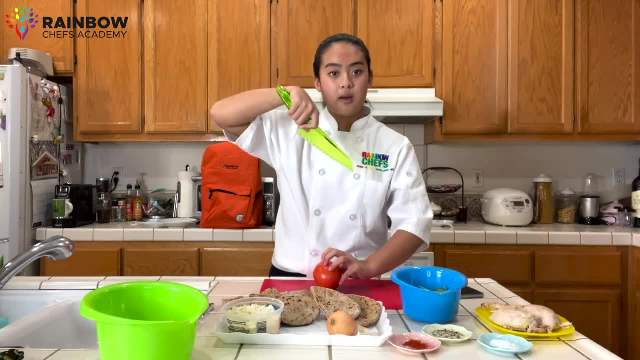 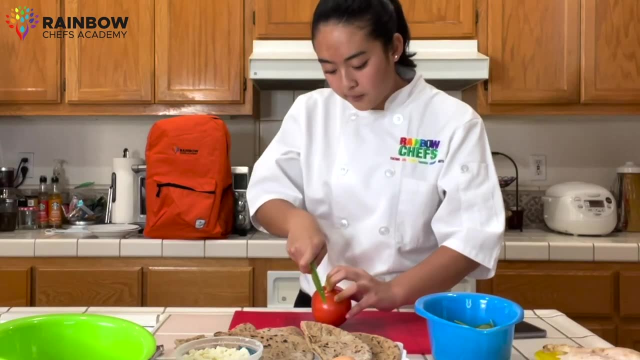 you want to use a wave-like motion, So we always want to start with the tip and then press down with the back of the knife. So, to start, we're going to cut off the stem, So we're going to place it in the middle of the knife And, using wave-like motions, we're going to slice down. 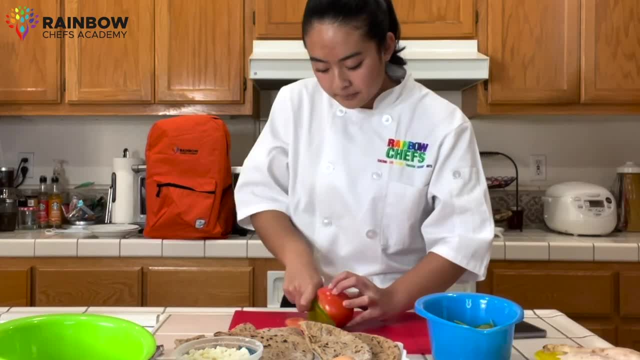 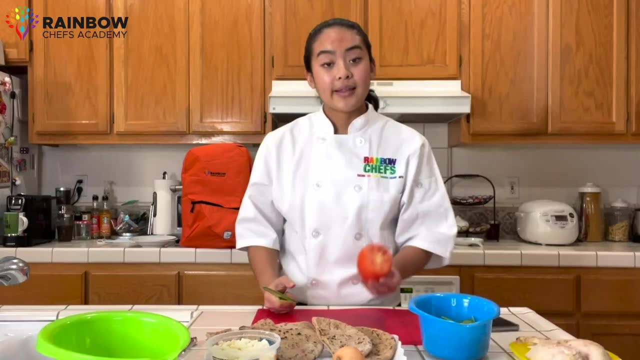 again until it goes all the way through the tomato. Make sure to cut as close to the stem as possible with us, so that way you're not wasting any tomatoes. You could dispose this Next. we're going to cut in half, So we're going to place the flat side that we've cut down And then we're going. 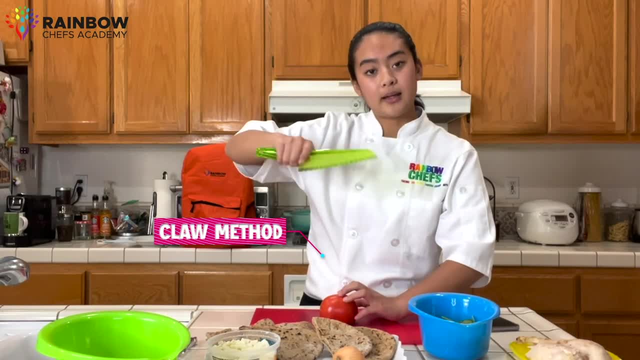 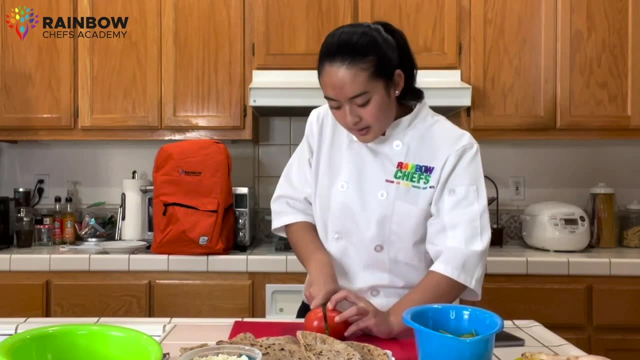 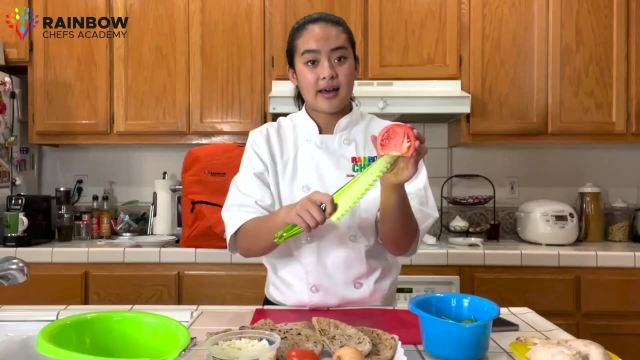 to use our claw pinch, grip, thumb and pointer finger gripping the knife, Wave-like motions right in the middle. And there you go. Perfect, Now we're going to place the big flat side down And we're going to cut this in half again: Claw pinch, grip, wave-like motions. 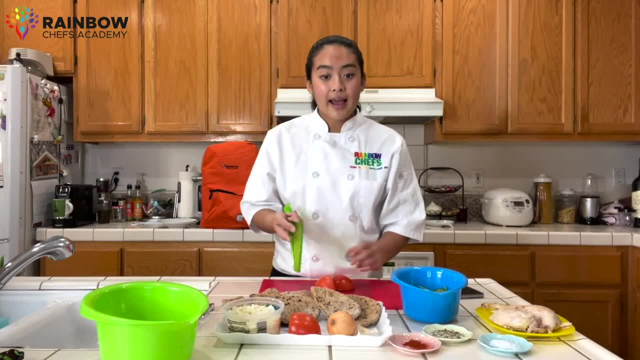 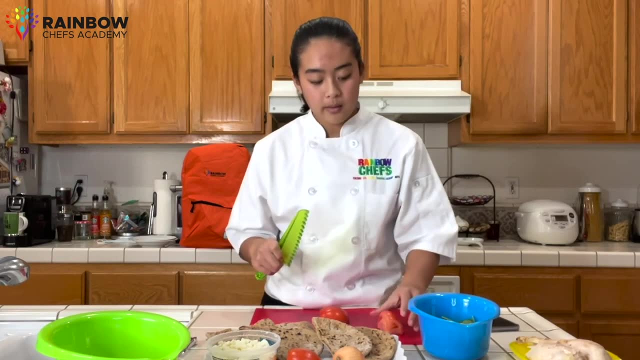 Perfect, Okay, from here we're going to begin dicing: So if you were to place one of the quarters down, face down, so that way it's flat and it's able, we're able to cut it. We're going to start by cutting slices. 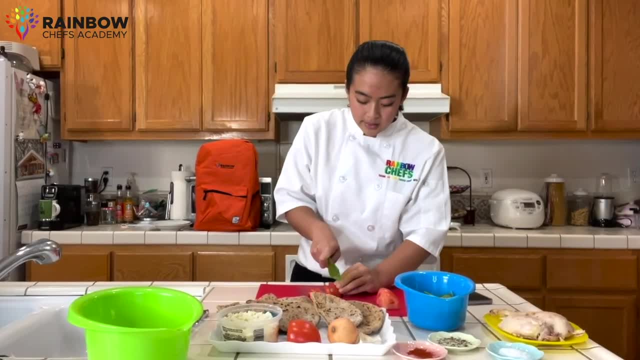 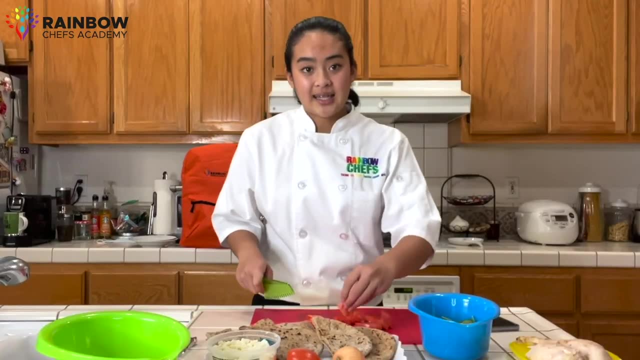 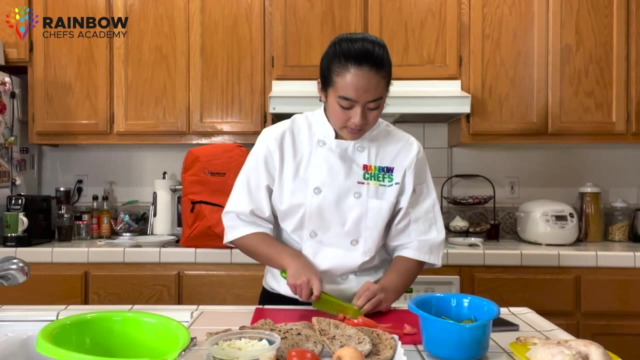 Using our claw, wave-like motions and our pinch grip, you should get slices just like these. Keep going until you get all your tomatoes done. After you're left with slices just like these, you are now going to be dicing them, So you're going to cut again using your claw and pinch grip. 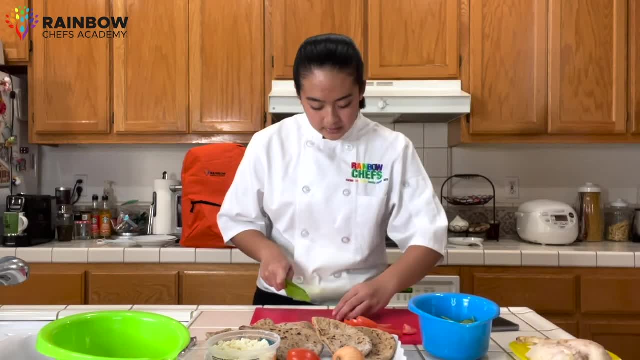 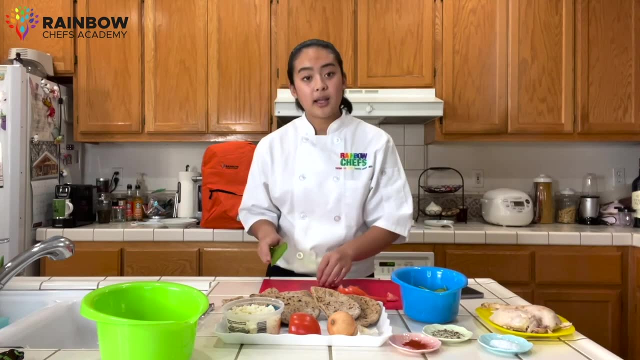 and wave-like motions. You're simply going to cut them into little cubes. You're going to make them almost bite-sized pieces so that way, when they bite into our chicken paint pocket, you don't get a huge bite out of them. You should get little cubes just like these. Continue to do this with the rest of your tomatoes. 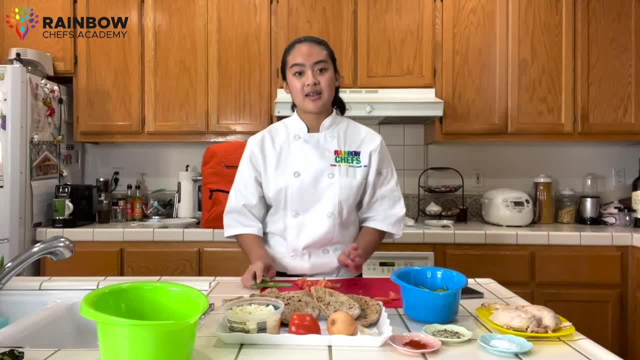 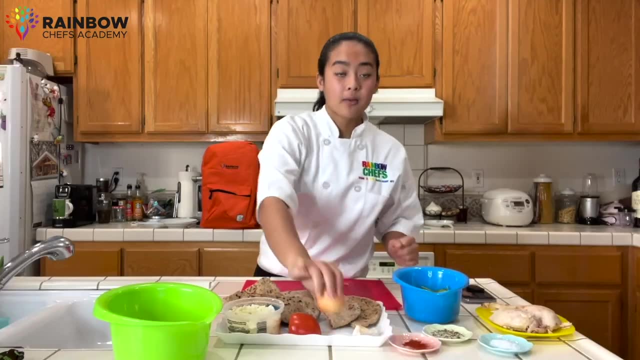 And when you're done, you can simply lift your tomatoes and put them into your small to medium sized bowl. Now that we've finished cutting our tomatoes, we're now going to start on our onion. So I took a really small onion because you don't want too much of it. 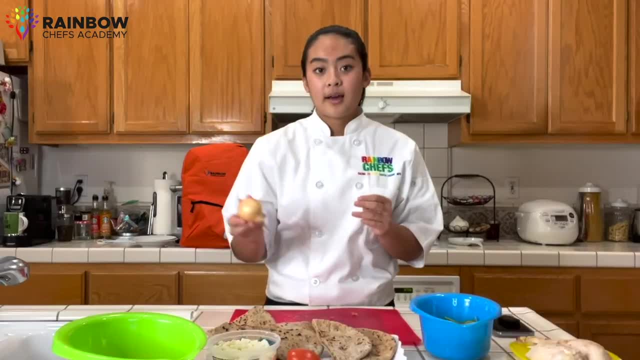 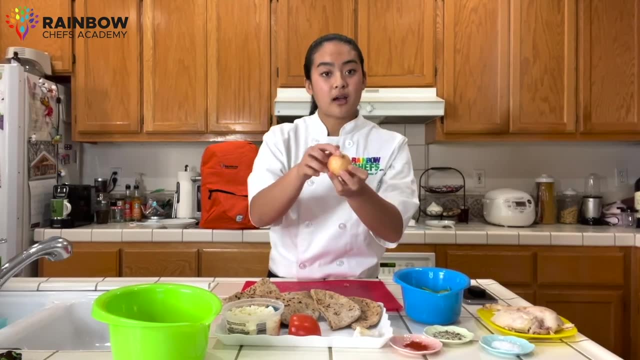 but if you have a bigger one, go ahead and use that. So onions do make you cry, but a tip is to not cut off this stem part that has the roots coming out of it. Feel free to cut off the top that has all the peel attached to it, but do not cut off the small part. That will prevent you from 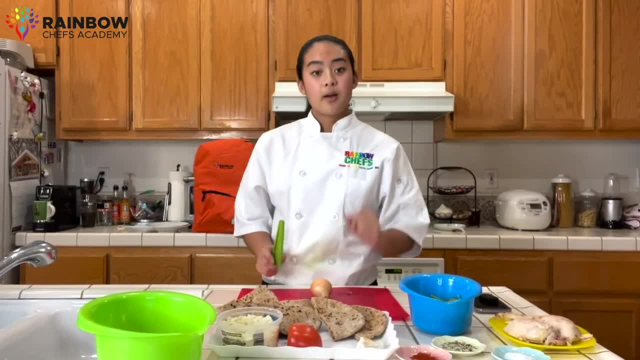 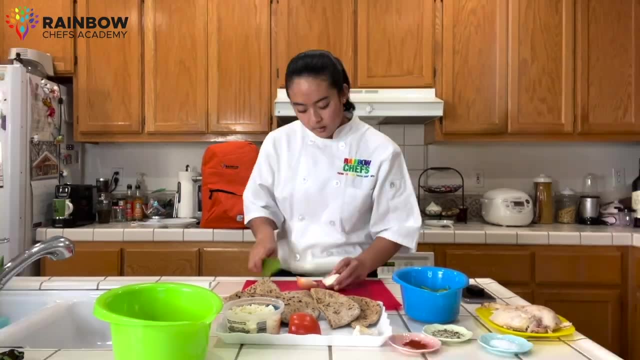 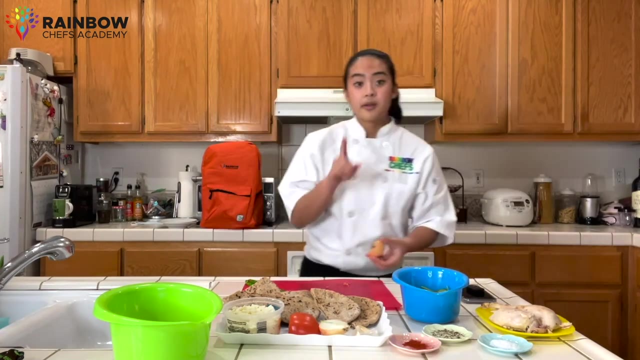 crying and your eyes being hurt. So we're going to cut this in half. So, with your claw and pinch grip, cut it in half, cut all the way through and then from there you can go ahead and head onto your garbage can and peel off the skin. You can actually cut it too, to kind of help you out. 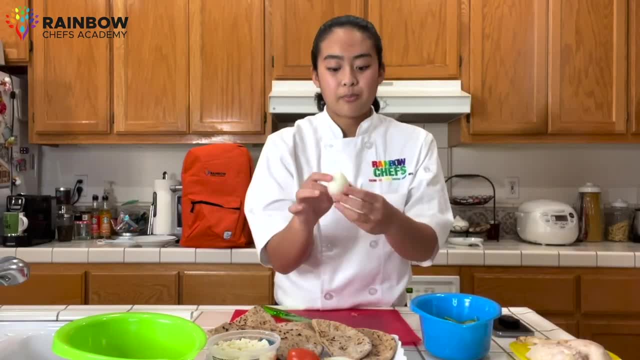 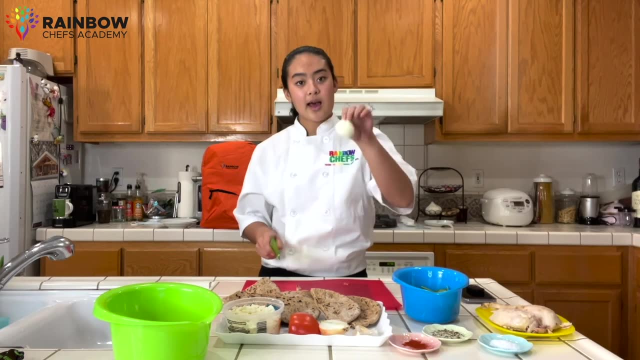 After you do this, you'll be left with the white onion: Perfect, nice and pretty. From there you're going to want to slice strips, but keeping not going all the way through, so that way it stays together as one pod. So you're going to. if you look at the onion, there are little. 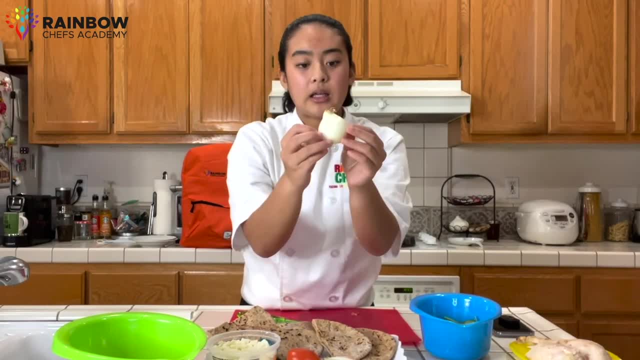 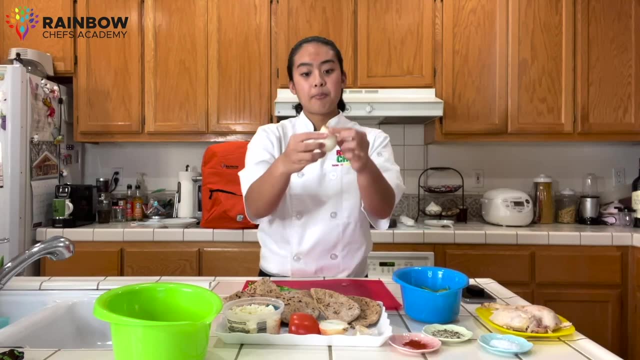 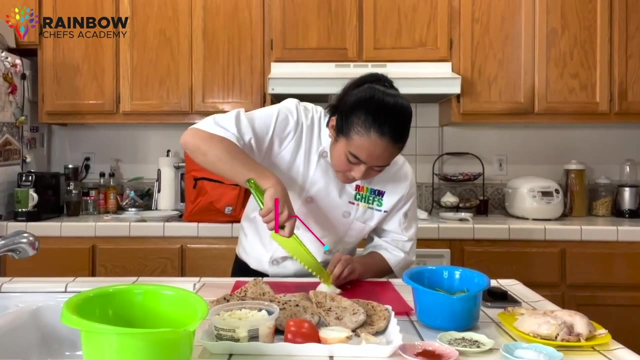 lines that go across the surface of the onion. You're going to want to cut through those, but remember, do not cut all the way through. You want to cut until you reach the tip of the border of the onion. So, using the tip of your knife, the pinch grip and your claw, holding the knife steady. 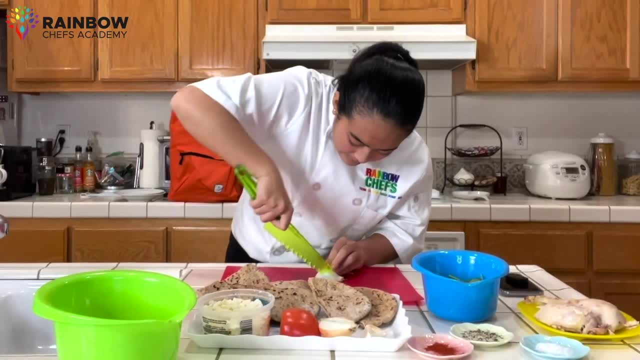 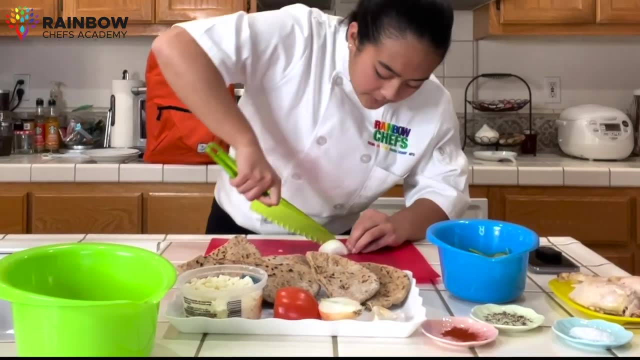 and slicing through just like that. If you need help with this one, kids, make sure to ask your parents. They'll be more than happy to help you. But if you've got it, make sure you're just very careful with the knife. We don't want any fingers to be cut off, and make sure to use your brick. 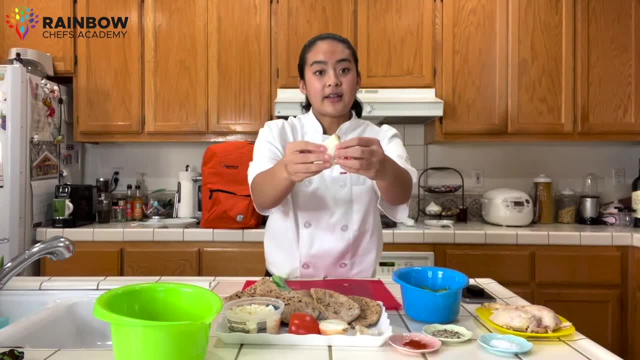 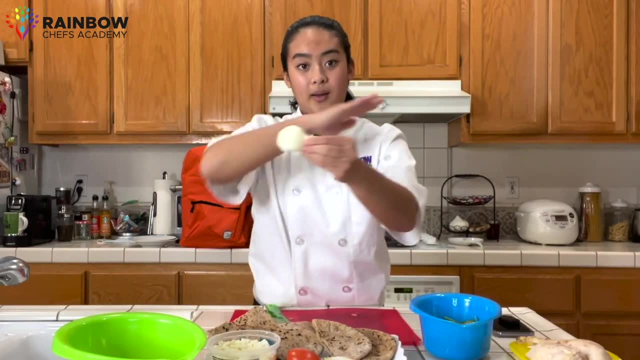 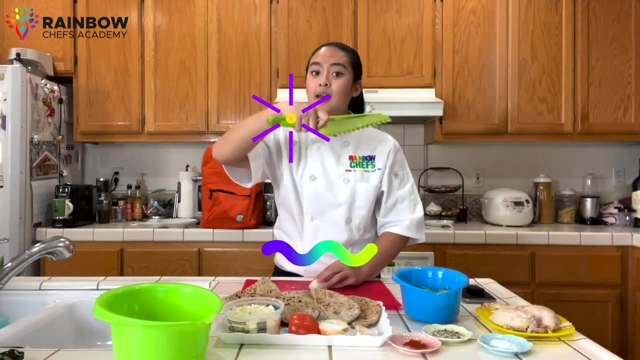 claw. So after you cut it into strips, as you can see mine, I cut it vertically, which is long ways down. You're going to turn it horizontally, which is long ways to the side, from left to right, And you're going to dice them. So you're going to slice down using a wave-like motion pinch grip. 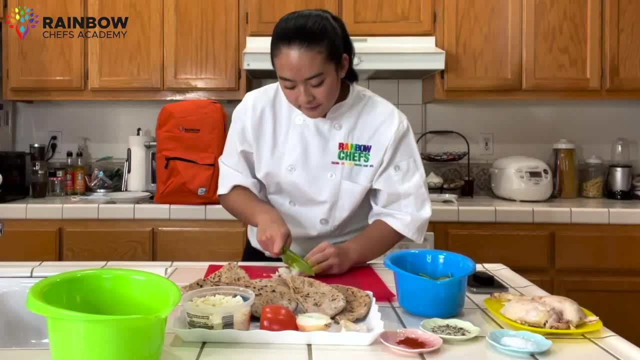 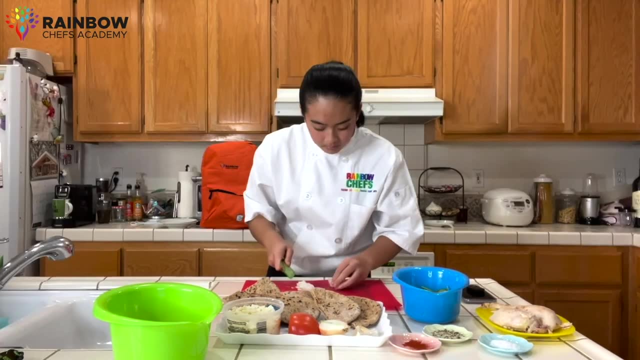 claw. You got it. Make sure to cut really thinly and that way we have the onions being really, really small and tiny and we won't get a huge bite of onion in our chicken feet pocket. Perfect, I'm going to throw this down away. And then we are left with our beautifully cut onion. 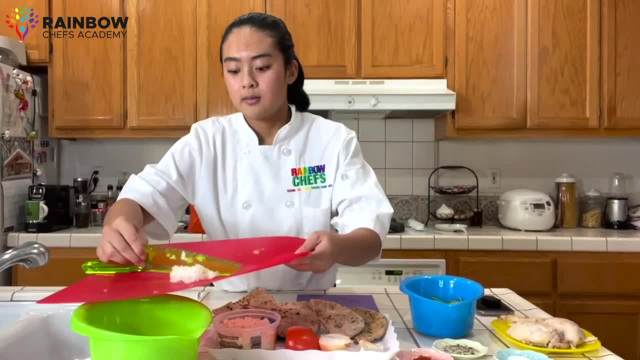 You can add this to our tomato mixture. Now that we finished cutting our tomatoes onions and we placed them in a bowl, we're going to put them in a bowl and we're going to put them in a bowl and we're going to 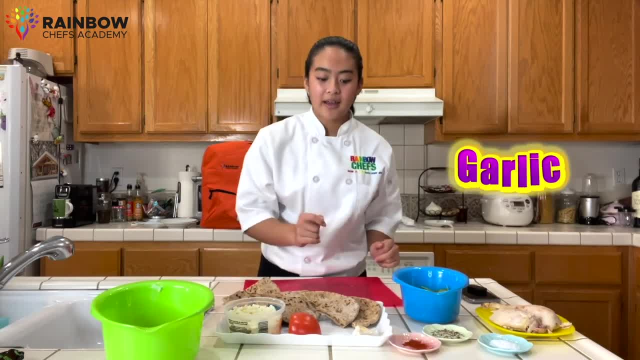 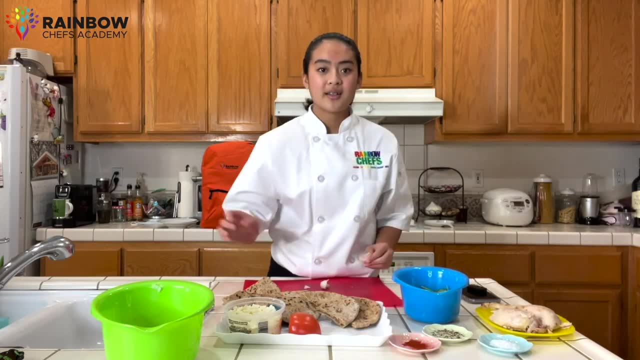 put them into our mixing bowl. We're going to now learn how to make some garlic. So, as you can see, garlic it's a very, very small thing to cut. It could be very hard, but I assure you it's not as 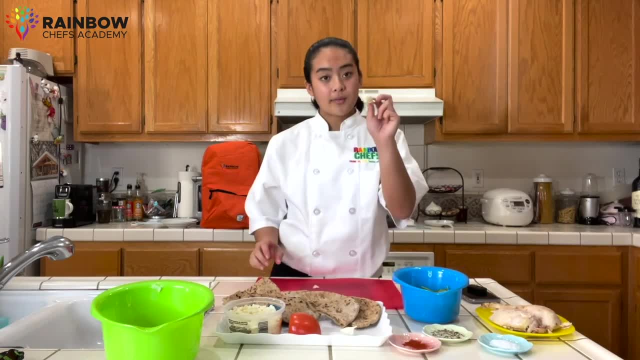 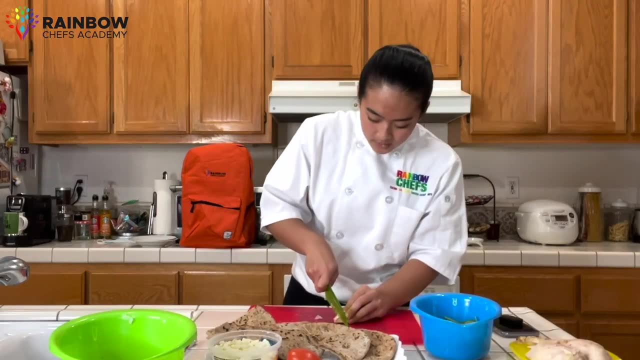 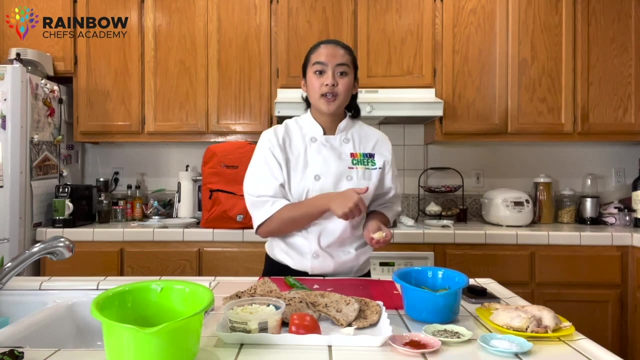 hard as it seems. So you're going to grab your one clove and you're going to use your pinch grip and your claw to cut off the stem. Wave-like motions again slice down And then, once you see all of the peels coming off, you can go ahead and head over to your garbage can again and peel off. 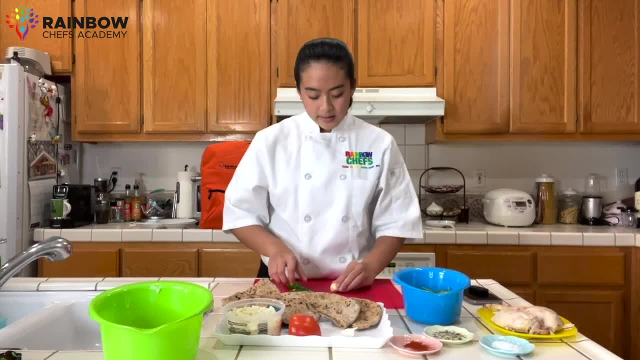 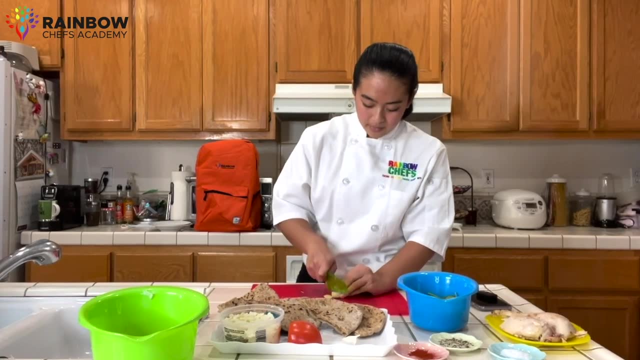 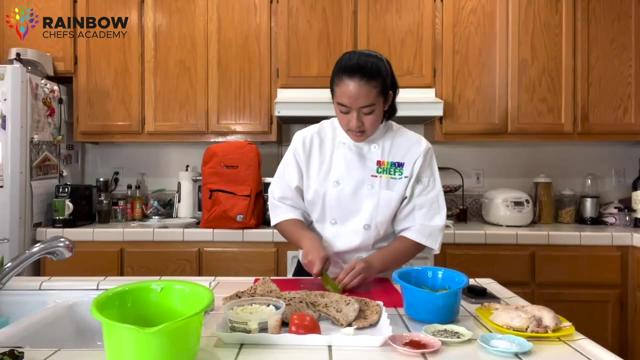 all the skin, like we did to the onion, Like we have here. you're going to now begin to dice it. So you're going to slice it using your claw, pinch, grip and wave-like motions and stalling back and forth, So that way you get thin slices of it first And then for mixing. 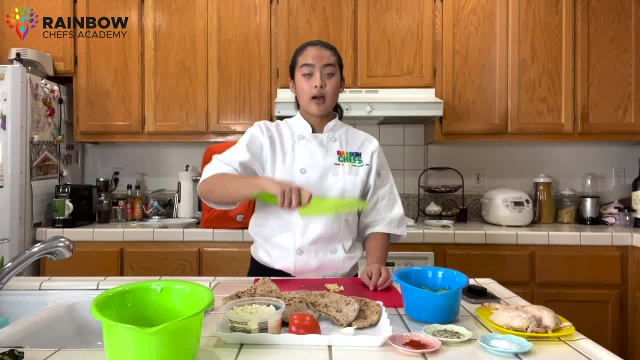 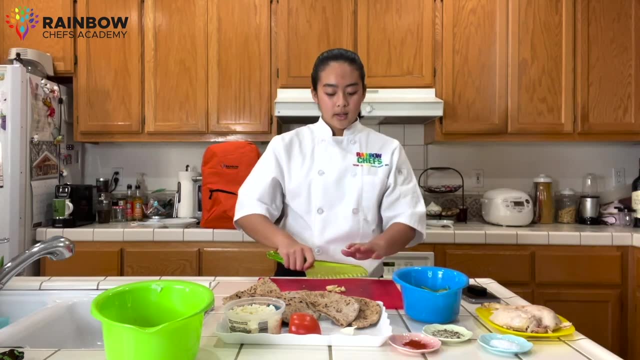 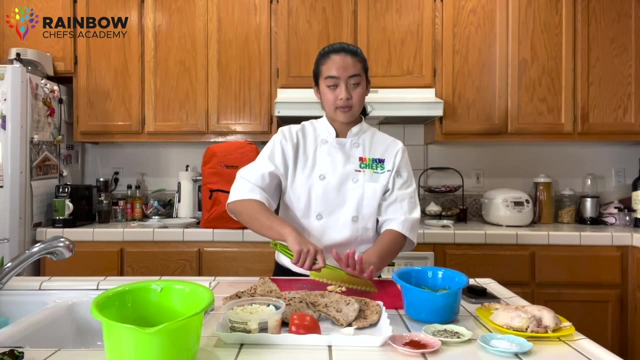 what you're going to do. you're going to still use your pinch grip and your grasp on the handle, but instead of using your claw, since the pieces are too small to hold, you're going to simply place your knife tip on the board. You're going to use your other hand, palm flat. 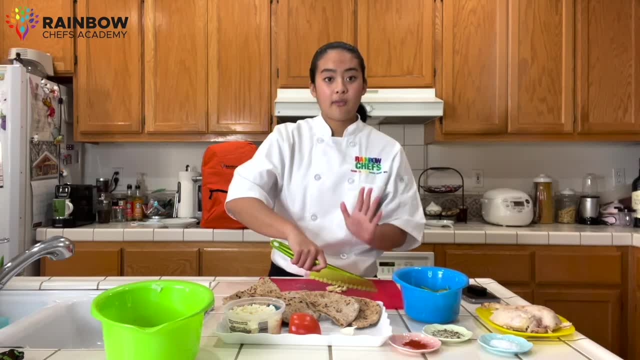 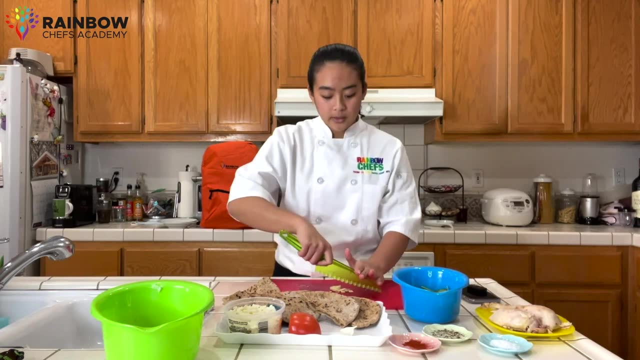 avoiding fingers to be curling because you don't want them getting under your knife dangerous. So you want to hold your palm out and you simply want to let your hand that is holding the handle do all the work. You're going to pump up and down, cutting really small pieces of the garlic. 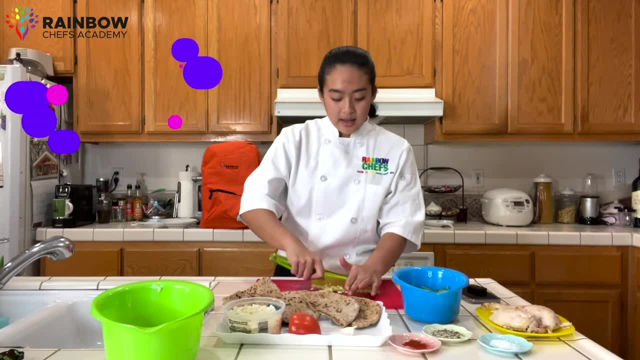 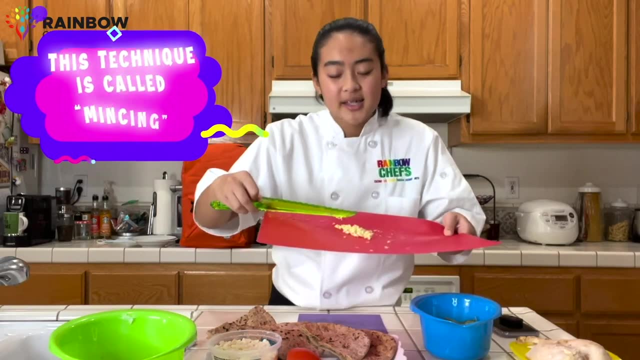 And continue to do this until they're all really small pieces, And this technique is called mincing. As you can see, I finished mincing. Our garlic is doing super, duper small pieces, And now we're going to add that to our medium. 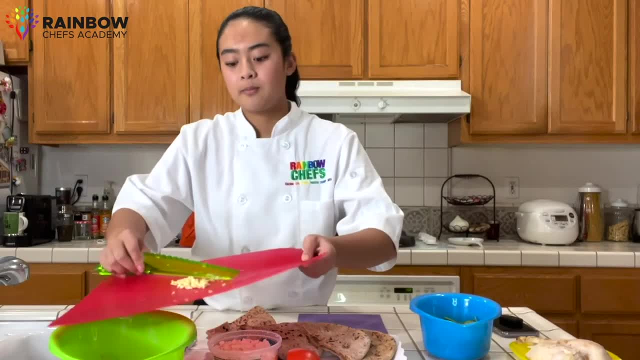 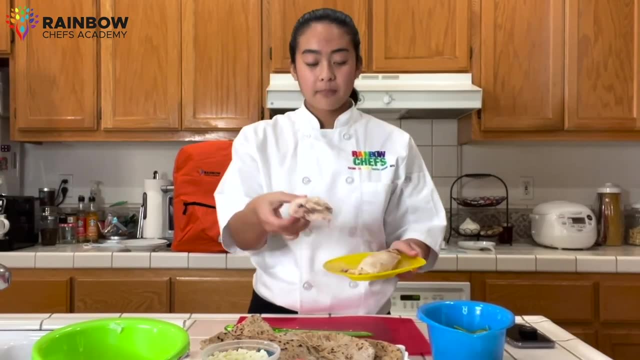 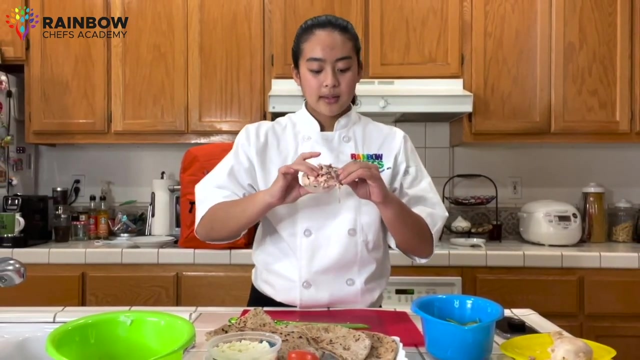 to small mixing bowl with our onions and tomatoes. Now we're going to move on to our main thing: chicken. So you're going to grab a piece of chicken. This is the breast. like I mentioned before, It has no bones in it, or ask your parents to extract the bone, But then it makes it super. 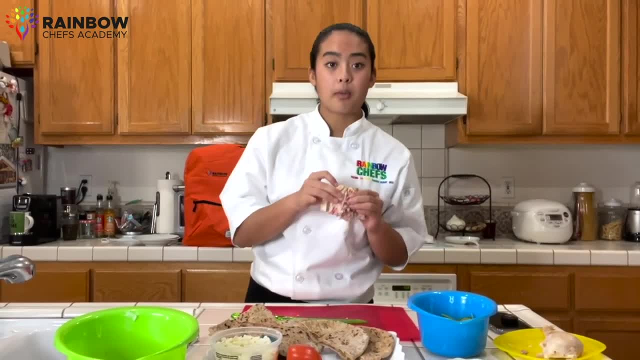 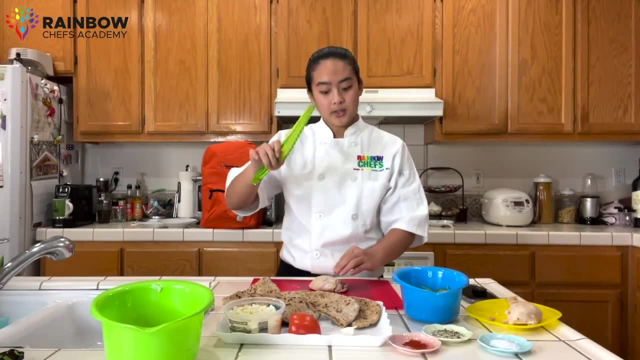 easy to cut. just because it is all meat. There's no bone that will mess with your knife and you can cut around it. So you're going to use your knife pinch grip and you're going to want to dice it. So, again, we're going to cut slices, then we're going to dice it, So holding it vertically. 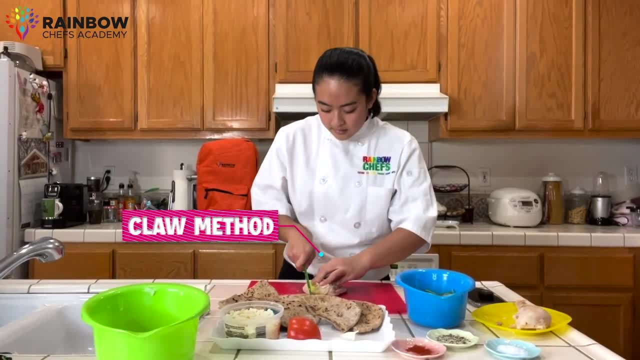 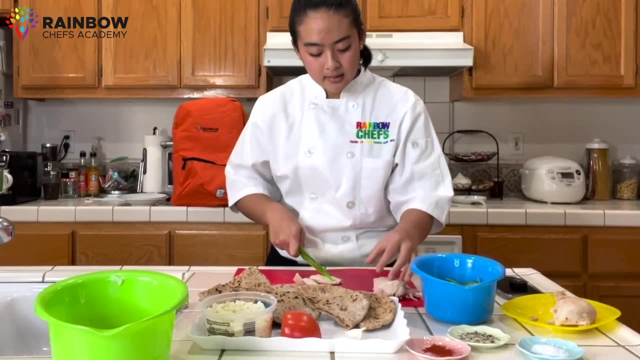 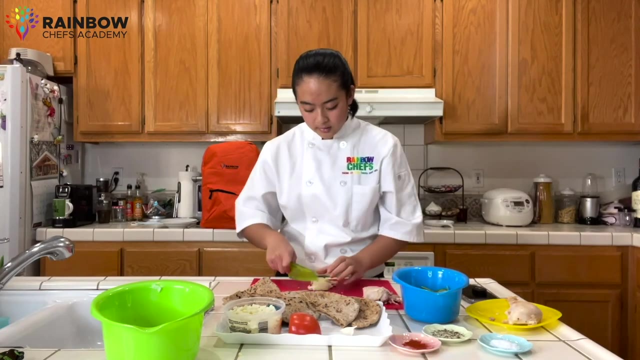 like this, up and down. remember, We're going to cut down using wave-like motions, our claw and our pinch grip- I'm going to actually separate this and that makes it a little bit easier for me, cutting this into strips, just like this, And then we're going to turn them horizontally or left to. 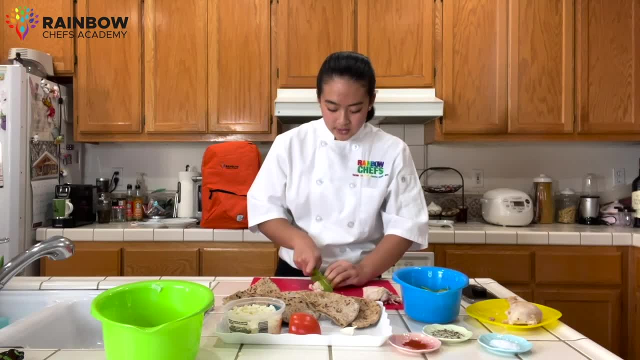 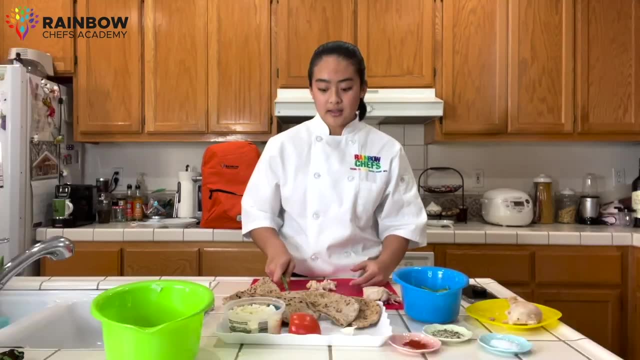 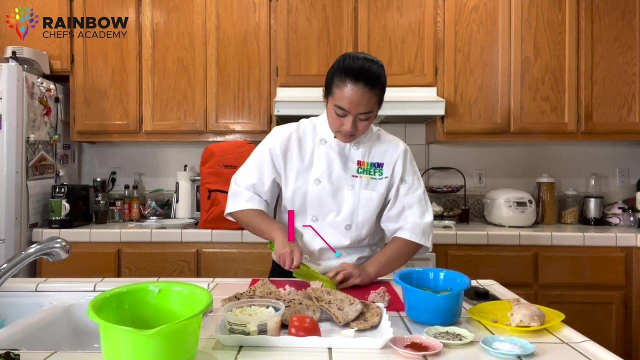 right and we're going to cut or dice the chicken. After doing that, you'll be left with little cubes that are perfectly bite-sized. You want to have a lot of chicken. This is because they need to fill up all the pitas, but you use as much chicken as you would like. Again, using my claw and my pinch. 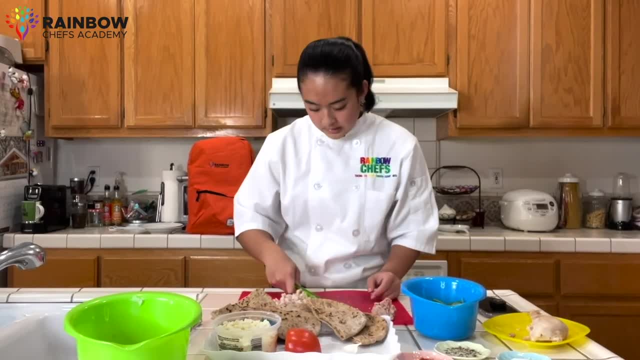 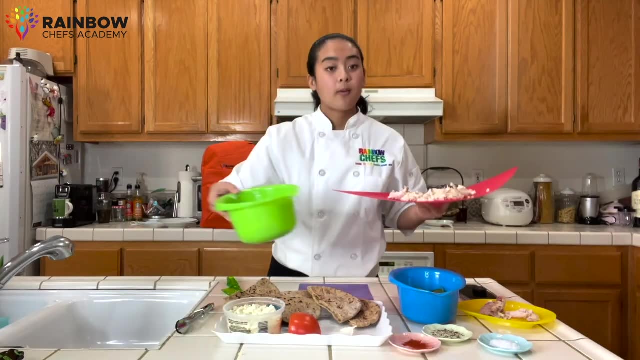 grip and my wave-like motions Keep going until all your chicken's done. Now that we've chopped all of our chicken, we're going to add it to our medium-sized mixing bowl, And then we're going to add our onions, tomatoes and garlic. It looks like so good. You can smell the tomato. 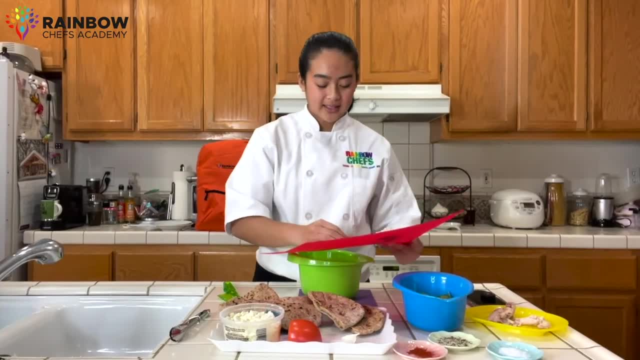 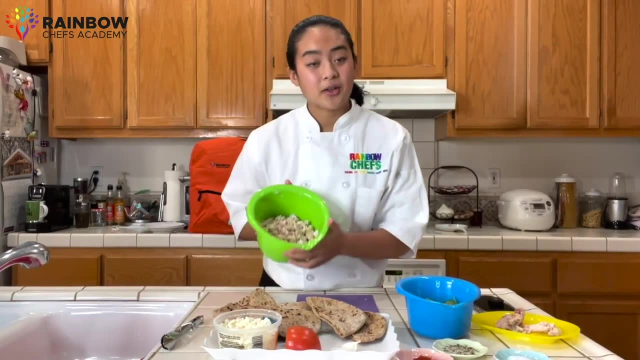 and the strong garlic. I love the little hint of onion. Now that we're done with the cutting board, we're going to simply put it in our sink. So, if you can see, this mixture looks insanely amazing, but we're not done yet. We have to add some seasoning to make it taste. 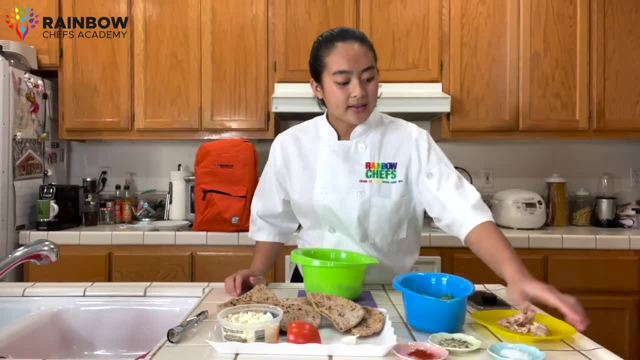 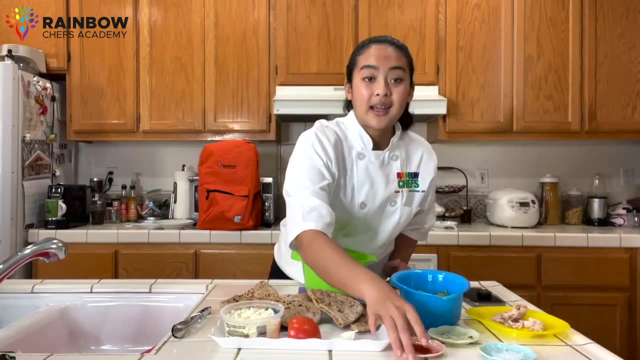 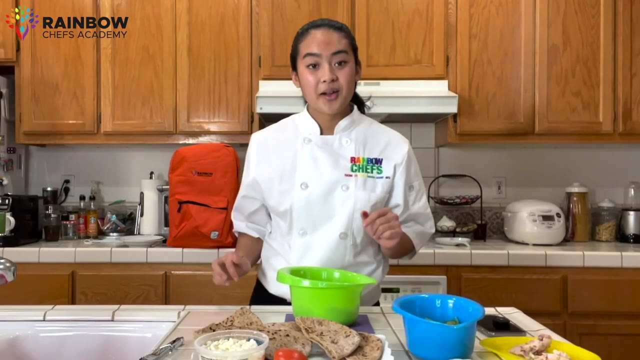 even better than it already does. So we're going to add some salt, We're going to sprinkle a little bit in Some pepper- This is freshly ground- And a little bit of paprika for some heat. But feel free to skip this if you wouldn't like it a little spicy. I'm quickly going to go wash my hands. 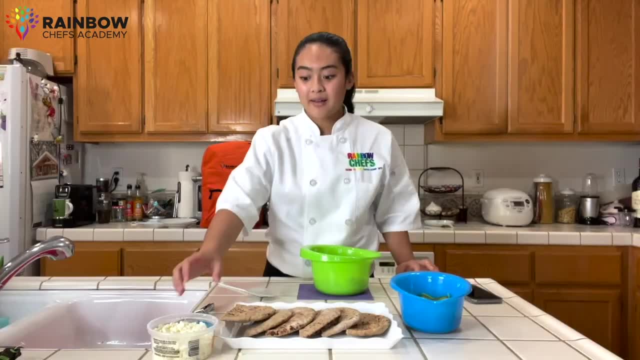 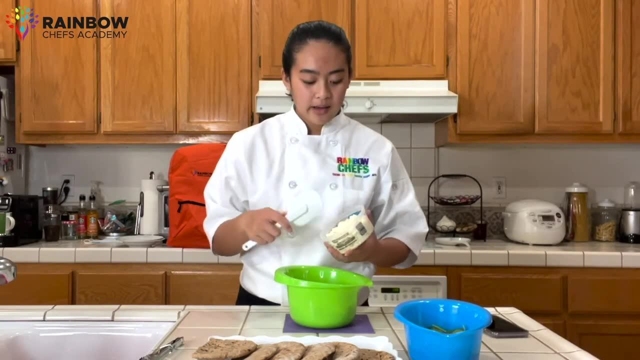 so I'll be right back. Now that I've finished washing my hands, I'm now going to add a little bit of feta cheese into our mixer. Feta cheese is a little sour, but it's also really tangy. I really 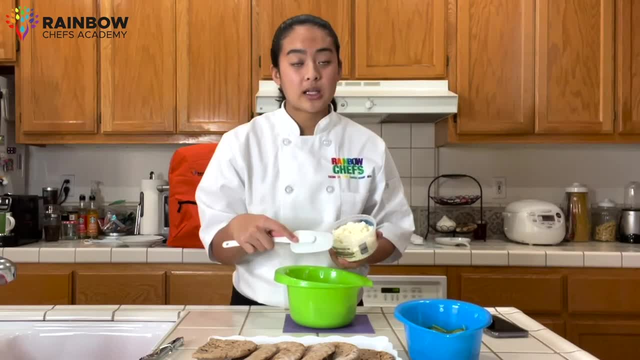 like it. But if you don't like it, feel free to substitute this out with regular shredded cheese or anything else that you would like Or don't like it. But I'm going to add a little bit of feta cheese And then I'm going to add a little bit of tomato paste. I don't add it, all, It's. 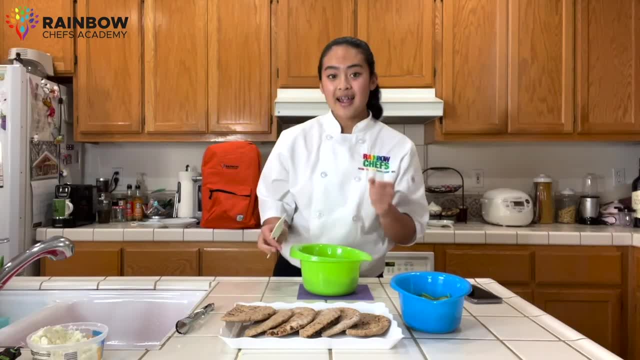 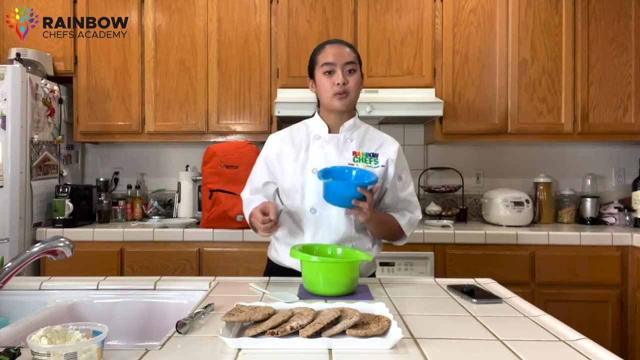 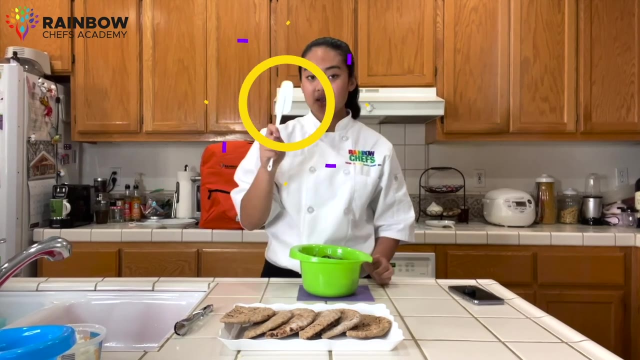 joke to you, So I'm going to add a little bit in. Next, I'm going to sprinkle in a few leaves of spinach. I washed this, but if you get it from the store, make sure you give it a little rinse before you use it. Put that into our mixer And then, with my spatula, I'm going to give it a little.